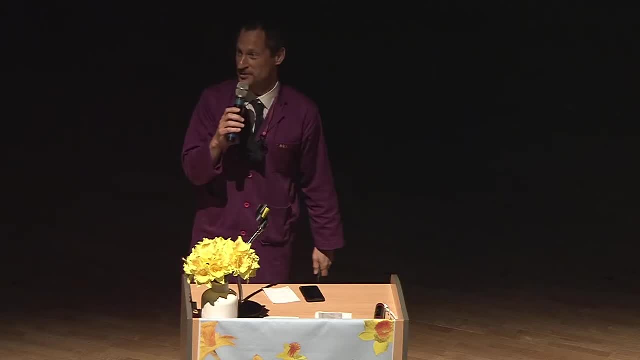 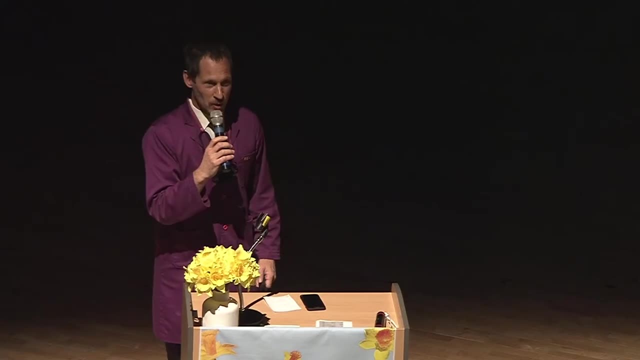 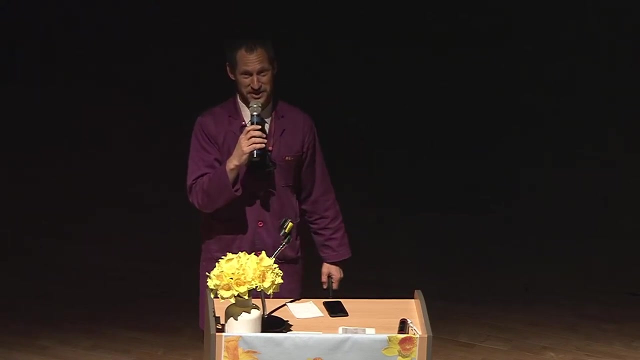 So, as part of the physics enrichment week, I want to talk to you this morning about two linked topics in astrophysics which were, not all that long ago, not even considered part of serious astrophysics or serious science at all. And they are exoplanets, which means planets that are not part of our solar system, planets that go around another sun, another star, somewhere in the galaxy. 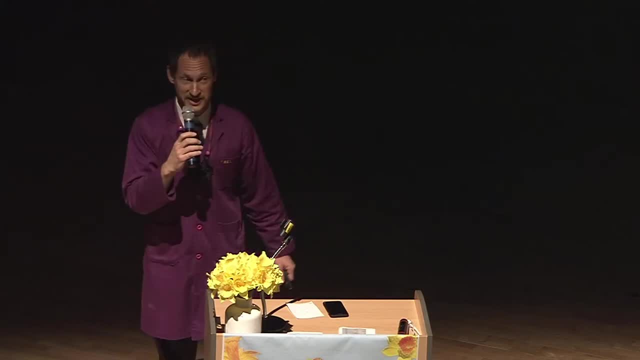 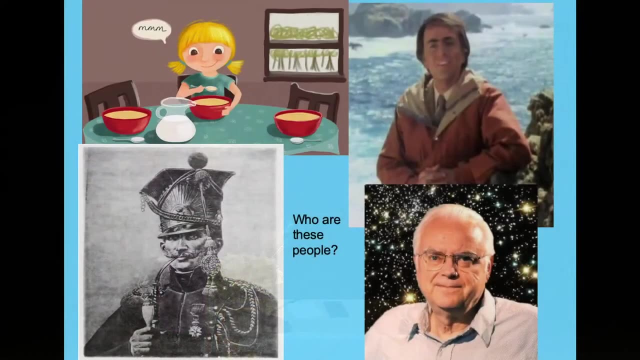 And the search for extraterrestrial intelligence, or SETI, looking for aliens. Okay, Right, We're going to mention at some point during this talk these four characters, Okay, And I'm sure you can recognize at least one of them. 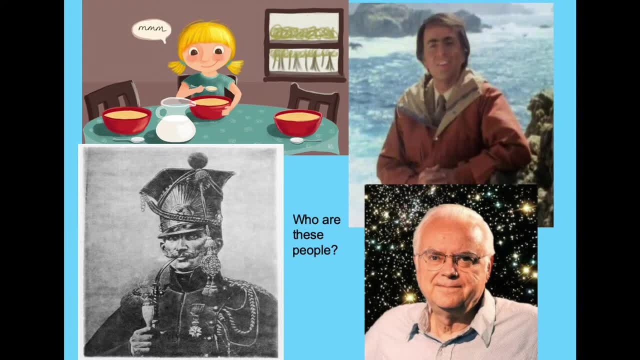 That's Goldilocks up at the top with her bowl of porridge, which is not too cold and not too hot, but just right. The top right is a very famous American physicist, astrophysicist and science popularizer called Carl Sagan. 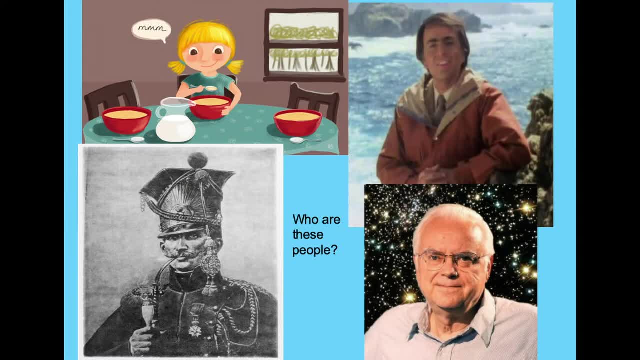 He's dead now. He died just over 20 years ago, But he was the prime mover behind establishing the search for life elsewhere in the galaxy as a serious thing for scientists to do Down the bottom left. Actually, we're not quite sure if it's a real picture, but that's a chap called Nicolas Chauvin, who was French. 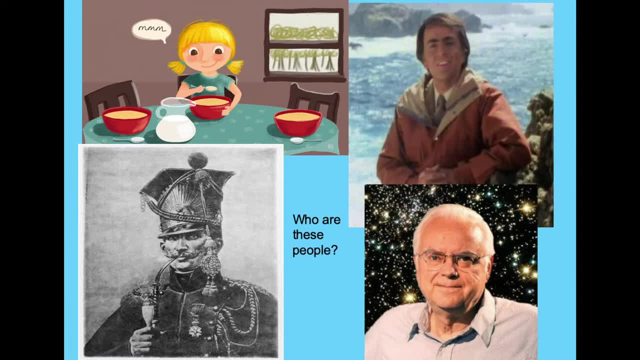 And he gave his name to the word chauvinism, which you may or may not know. We use it particularly to talk about male chauvinism, In other words, men thinking that only men can be good at something and women should be staying at home, not working. 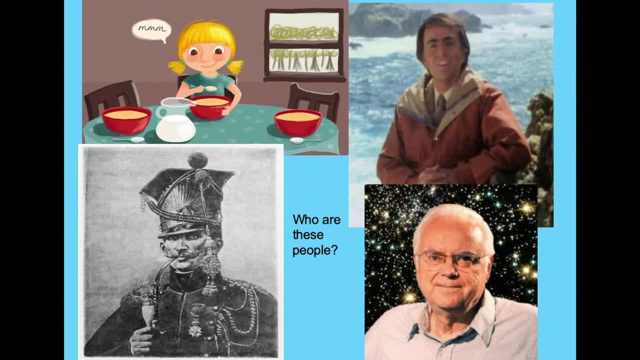 The terribly old-fashioned views that we do not hold anymore. But we use the word chauvinism more generally as well to talk about any kind of prejudiced ideas, The idea that, oh, I do this this way, so it must be the best way. 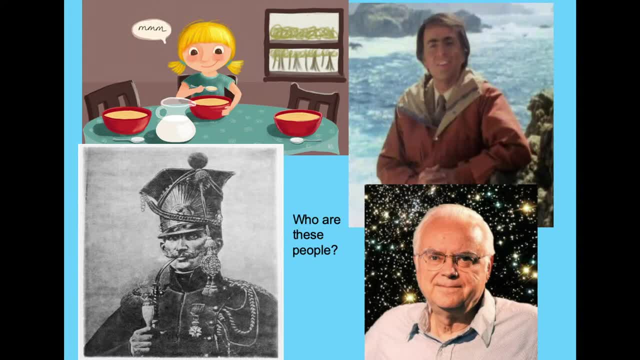 This applies to me, so it must apply to everyone else. We'll be talking about that idea too, And down there in the bottom right is a chap called Frank Drake, also an astrophysicist, And he came up with a well-known equation which is used when we're considering looking for extraterrestrial life. 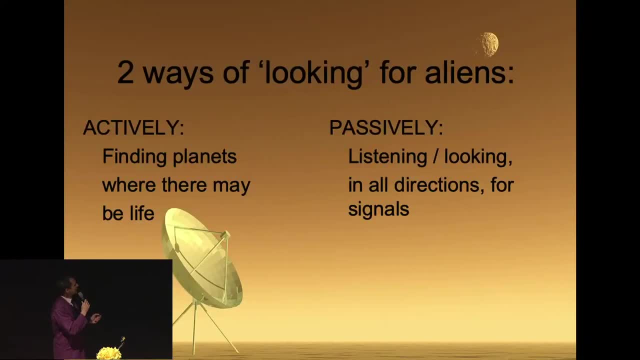 We'll be looking at that as well. There isn't a test, Don't worry. Okay, So there are two ways, really. There's the first way of looking, if I can use that word, looking for aliens, And one is to actually go out and try to find planets around other suns. 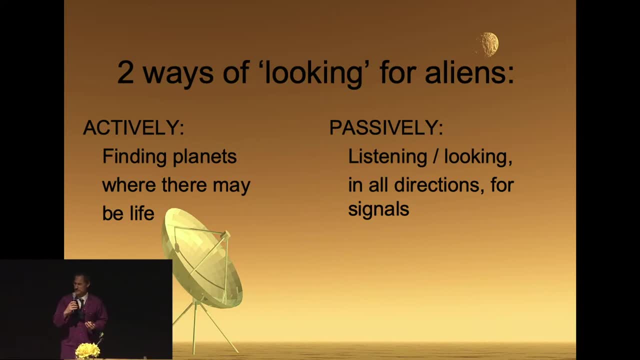 Because, as far as we know, that's the only way you can have life. Nothing lives on a star itself. Nothing lives on freezing cold asteroids hurtling randomly through the galaxy. Things live on planets, perhaps. And the second way is what we call the passive way. 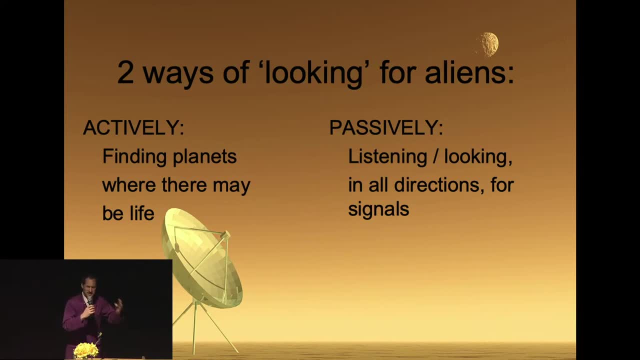 Which is, rather than actually searching in a particular direction or for particular kinds of planets around a star, is to sit here and listen, To build big dishes like satellite dishes, but not orbiting. You know, dishes sat here on the Earth. 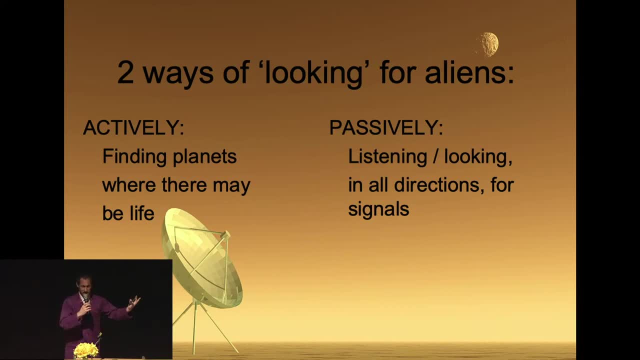 You can put them in orbit And analyzing the radio signals that we receive from all directions That come to us- And of course, most of that is noise. It's of natural origin, And scientists and computers automatically spend a lot of time trying to work out whether there's anything that could be artificial in these signals. 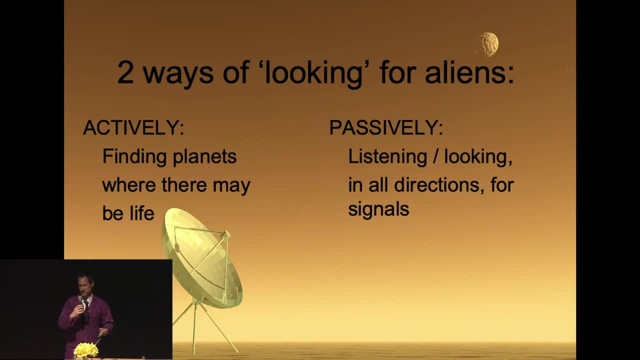 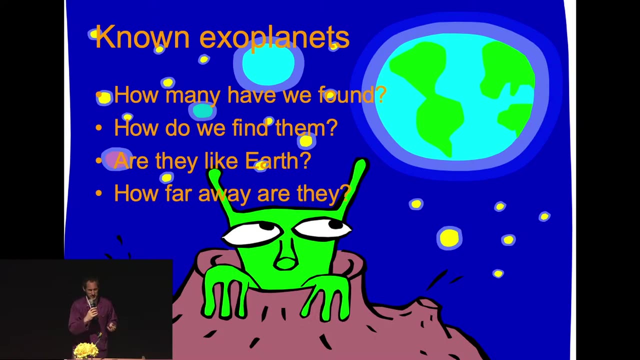 Anything that indicates hang on. that took intelligence to create that signal, So known exoplanets. As I said, it used to be science fiction. The first accepted data Hang on. that's definitely an indication that there is another planet out there. 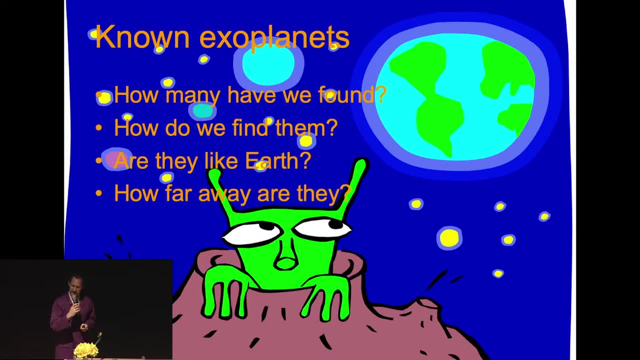 Was only in, if I get this right, I think 1995.. Okay, That's younger than most of your teachers, Most, several of your teachers, It's certainly younger than me. In other words, when I was your age, there was no known exoplanet. 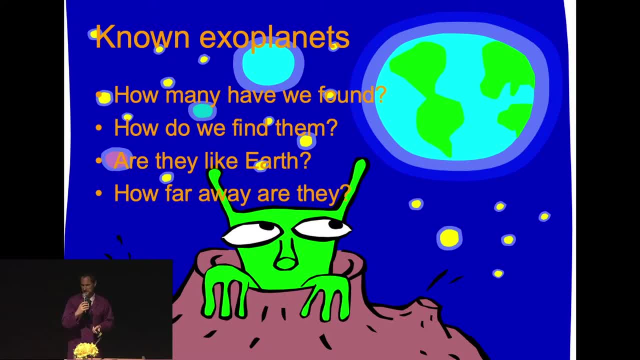 As far as anyone knew, the only planets in the entire universe Were Mercury, Venus, Earth, Mars, Jupiter, Saturn, Uranus and Neptune. Okay, And now that seems a tremendously parochial, closed idea. Why would other stars not have planets? 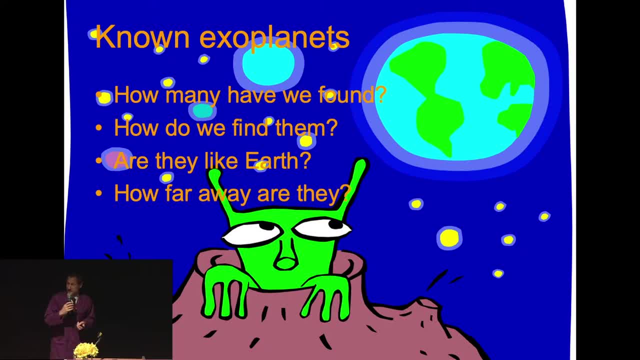 But that was the state of things. It's much easier to detect large hot planets, Particularly the size, for example, of Jupiter- Great, big balls of gas- Than it is smaller rocky ones like Earth. But the first Earth-like exoplanet was detected just over. 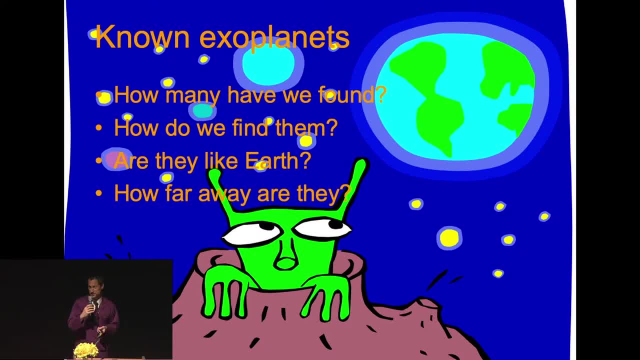 10 years later in 2007, So that's about as old as you. Okay, the idea that There are planets out there? there are definitely planets out there That are suitable for our kind of life. That's only the same age as you. 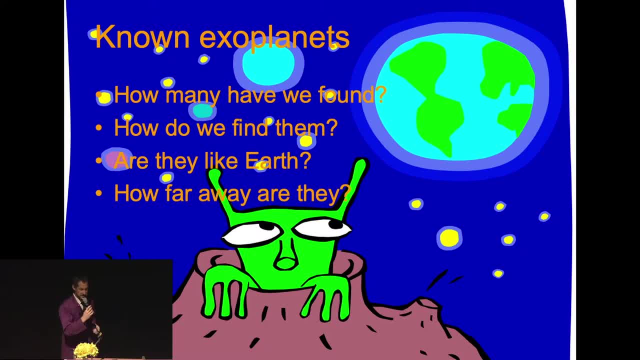 It's not an old idea, And now, as of a couple of weeks ago, last time I checked, We know about four and a half thousand exoplanets And there's no reason to suspect that that's it Okay. there are surely tens of thousands, hundreds of thousands of exoplanets out there. 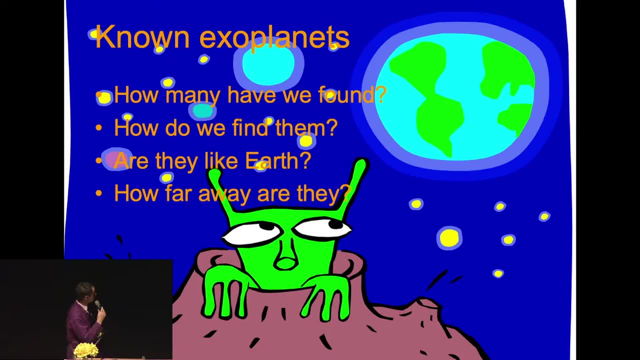 of thousands more, But that's how many we know of at the moment. I want to talk a little bit about how we find them. There are two principal methods and a couple of others which are used to find a few more every year that I'd like to talk about. And then we also want to answer the 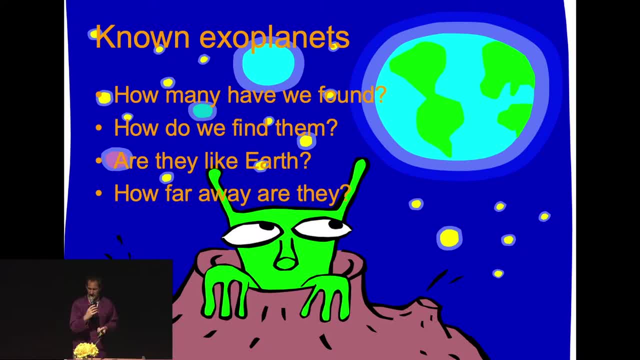 questions: how much like Earth are they And how far away are they? Is there any prospect, if we do find life, of actually entering into meaningful interactions with such civilizations? So it's not an easy thing to do. Stars themselves are extremely far away. 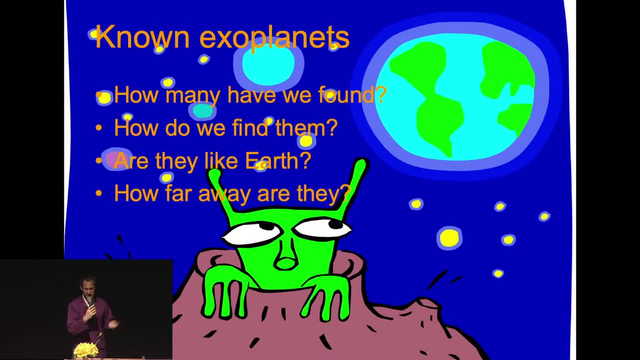 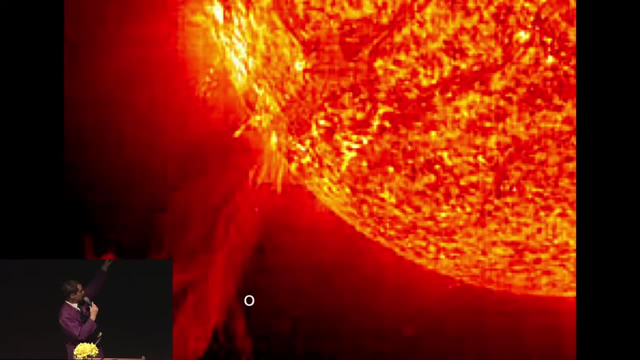 So, although they're huge, they're already just points of light in the sky, And a planet compared to its sun is something like that. That's actually our sun and that's how big Earth appears. So we're looking for something that tiny, orbiting an enormous hot ball, like our sun at distances. 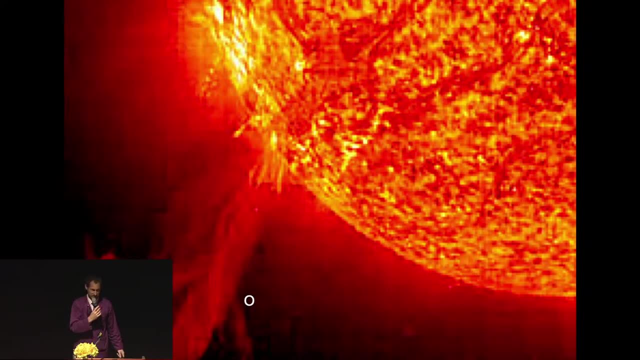 of several light years. A light year, just in case you didn't know- I think most of you do- is the distance that light travels in one year. Distance is speed times time: 300 kilometers per second multiplied by number of seconds in one year, And that's the distance that light travels in. 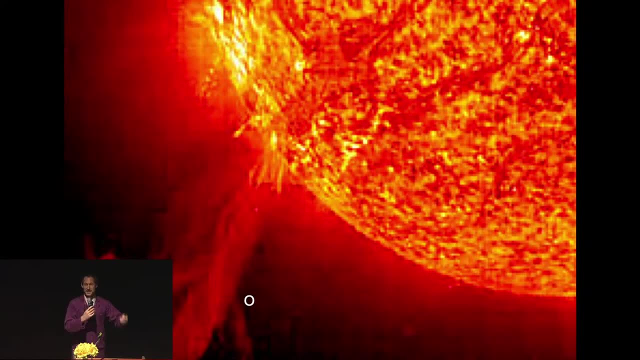 a light year, You get approximately nine and a half million million kilometers. That's one light year, Okay. The nearest other star to us is just over four of those away, So about 38 million million kilometers, And most are further away even than that. So we're looking for something. 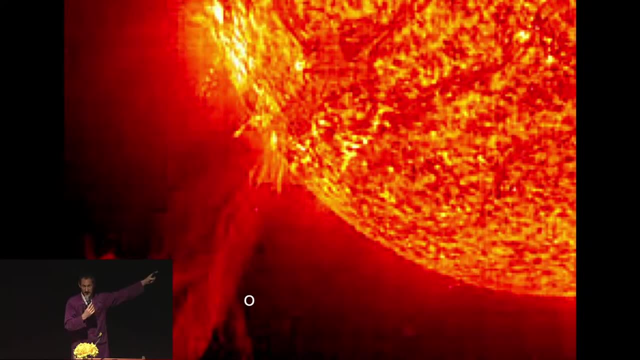 that tiny around something that vast, at these incredible distances. No wonder it's so big. It didn't happen until a few decades ago, right? So the two major ways in which we're able to detect exoplanets are called the transit method and the radial velocity method. Transit means: 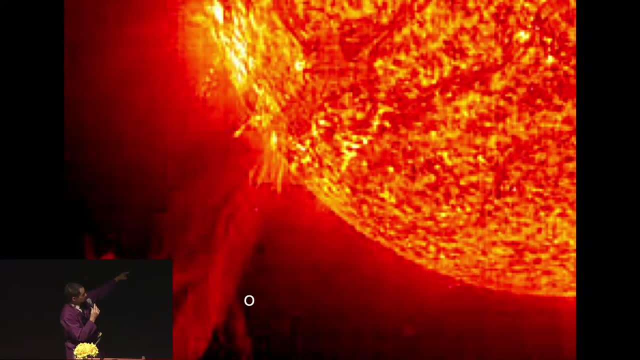 when a planet passes directly in front of its star, as we're looking at it, And that enables us to detect the very small drop in brightness. Okay, A planet is not a bright object And when it passes in front of a star, the brightness that we receive from that star. 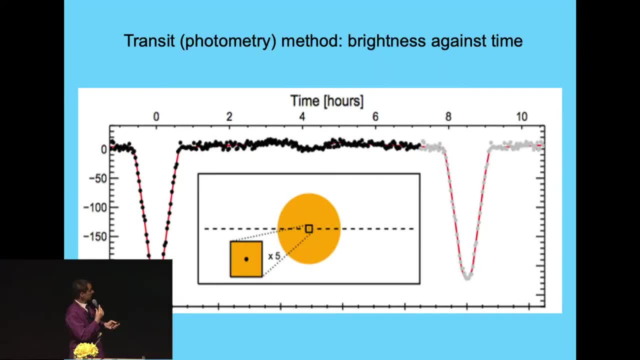 will drop just while the planet is going across. That's the kind of thing. It looks like a really significant drop in brightness, doesn't it? That's just been exaggerated for this graph so that you get the idea. It's actually only a very small drop. But there we are. We have our 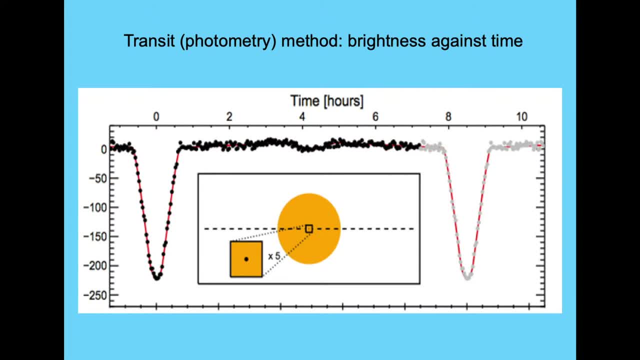 base level of brightness, The planet passes in front of the star and blocks out some of the light. Okay, And then, when it's gone past, we've got Our standard level of brightness again, And so we see from this not only aha, there is a planet. 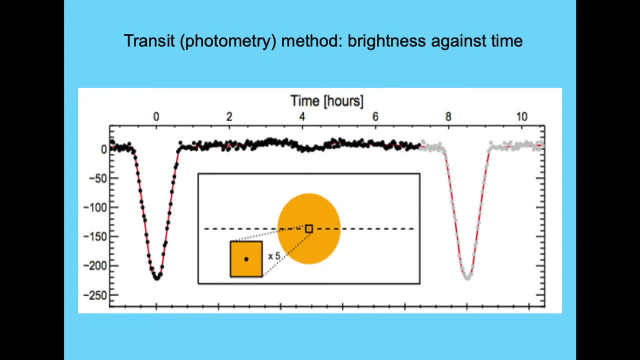 but also we can tell how long the planet is taking to go around the sun, because the period of the graph repeats. Now, obviously this method has limitations, And the most obvious one is it only works if the planet is orbiting around the sun in the plane that we are looking at it. If you've got 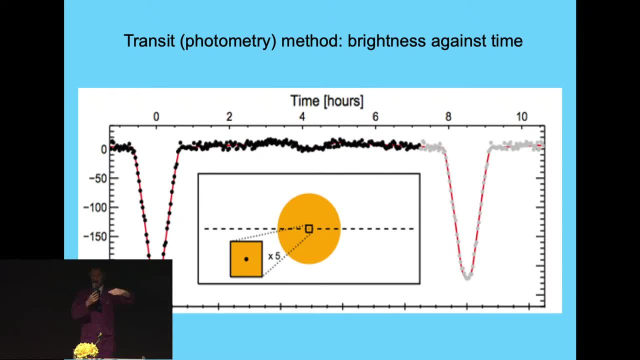 a sun here and the planet is going around like this. as we look at it, we're not going to spot it because it's not blocking any of the light, But this method works well. Okay, The majority of exoplanets that we found have been found using this method: analyzing the brightness, the transit. 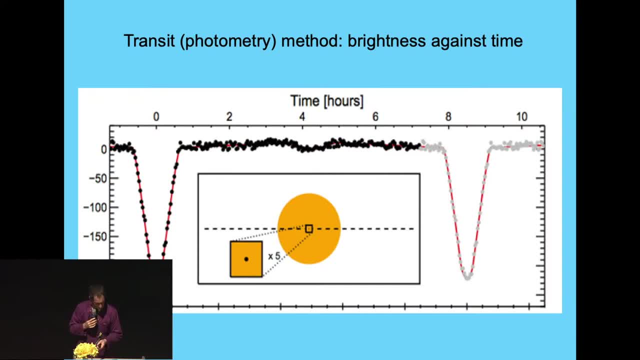 method. Okay, The other most important method- I haven't got a separate slide for this- is called radial velocity, And it has to do with the fact that a planet- again, although a lot smaller than the sun, is still a reasonably large mass- Okay, Large enough to be able to go around the sun, And 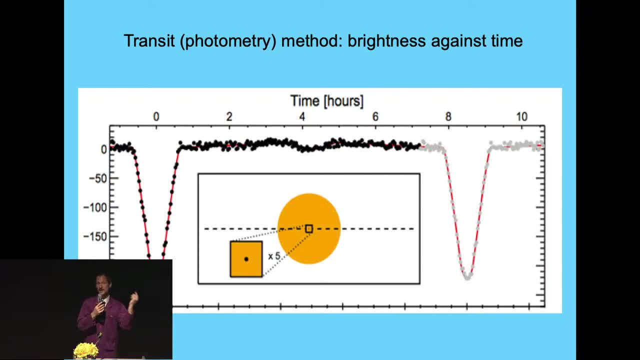 it has to have an effect gravitationally And we can actually tell as a planet orbits the sun from the wobble in the movement of that sun, of that star, due to the gravitational pull of the planet. Okay, So that's also enabled us to detect a reasonably large number of exoplanets And a 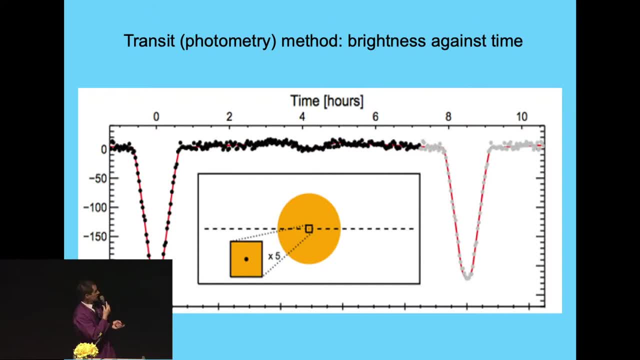 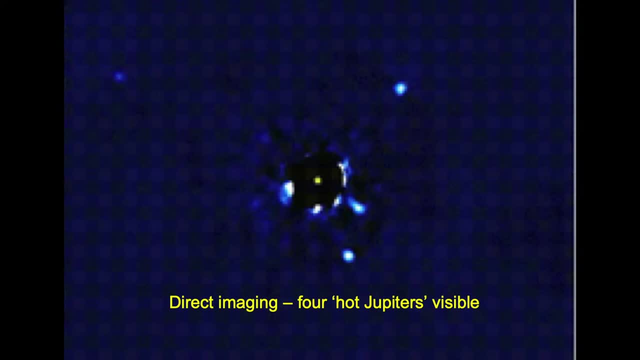 couple of other methods that just help us to detect a few every year. Just occasionally we're able to get an actual picture, Not invisible light. This is using infrared and it's been made up using false colors into a, you know, a visible light picture. But there's. 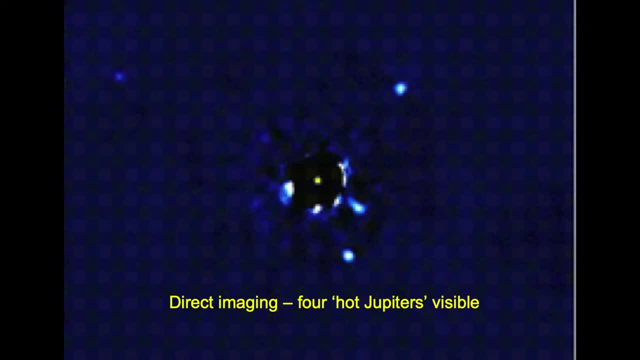 a star whose light has been mostly blacked out for the picture in the center there And then on the right one, two, three and one over. there is a fourth planet that we were able to observe in this star system just taking a straight out infrared photograph. Okay, This method works well for. 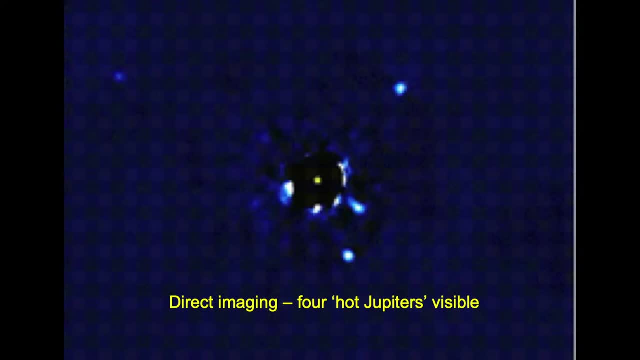 large hot gassy planets. Okay, It's called direct Imaging And the final one is called gravitational microlensing And it has to do with the mass of the planet, helping the star to focus light from stars that are behind it. Okay, In a particular 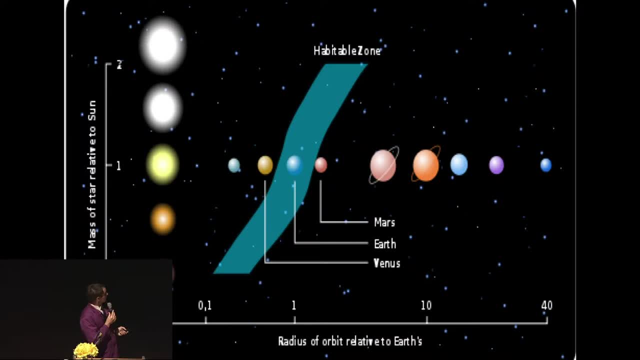 way, Right, Okay. So the question now, if you're interested in the looking for alien life side of things, becomes not just: okay, we found X, So planets, but is life likely to have arisen on those planets? And we bring in the idea of what. 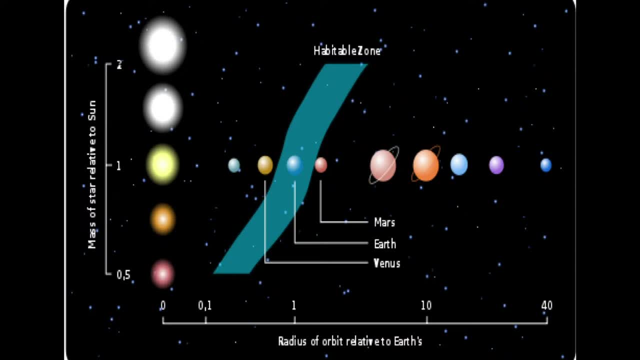 we call the Goldilocks zone- This is why we had Goldilocks on that slide earlier- or what scientists, perhaps a bit less informally, call the habitable zone, And that has to do with where water can exist. As far as we know at the moment, water is necessary for life. So in our solar 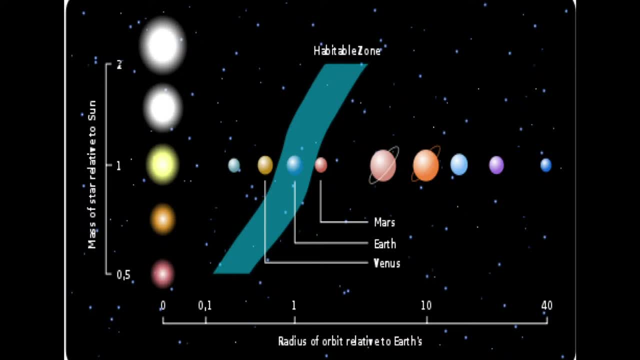 system. as you can see, Earth is slap bang in the middle of the habitable zone. Okay, Water exists naturally on Earth. Okay, In fact, we're so perfectly in the middle that water exists naturally as a solid and as a liquid and as 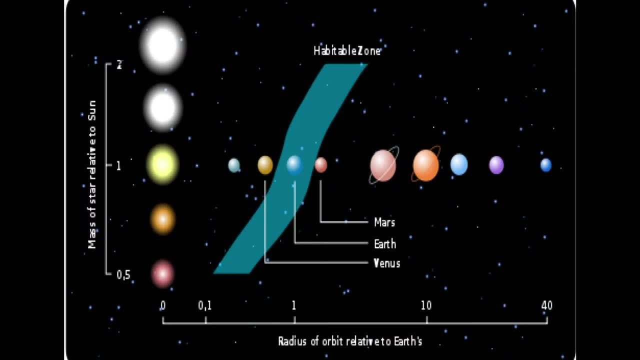 water vapor on our planet, Okay. But if you get too close to your sun, it's too hot, Okay, And water can't be liquid. It'll only be vapor if there's any at all. If you get too far away, you're going to 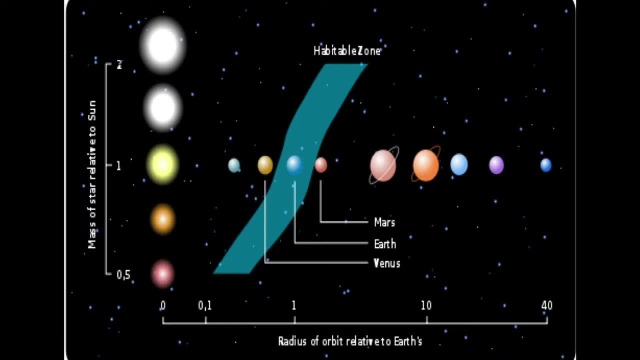 be too cold, Okay, And if there's any water, you're going to be too cold, Okay, And if there's any water at all, it's going to be solid. So we say, righto, this is the habitable zone. And on the 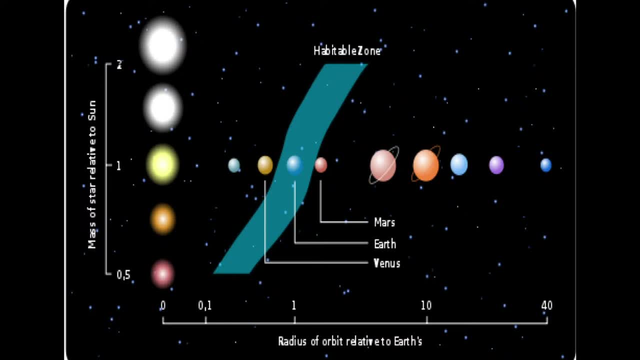 left, you can see pictures of suns of different brightness And, of course, if you're orbiting around a smaller sun, then this Goldilocks zone, or the habitable zone where water will be liquid, is closer in. Okay, Because the sun isn't heating up greater distances so well. If you're orbiting 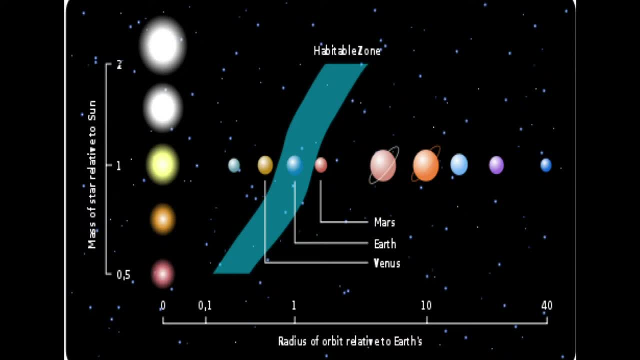 around a larger, more powerful sun, then the habitable zone is further away. Okay, But as I mentioned earlier, this is what we call a chauvinistic attitude, perhaps Just because on the only planet where we know there is life, which is Earth. okay, life requires water. Can we conclude? 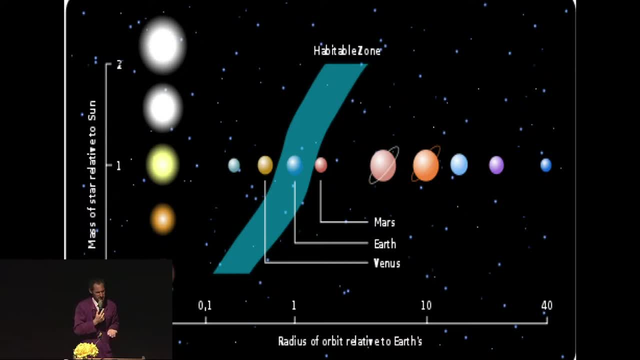 therefore, that life must rely on water. Is it impossible for life to have arisen on another planet, somewhere in the galaxy, where there is no liquid water? We can't possibly say for 100% certain that that's the case. We don't even know that life has to be based on proteins. Okay, We don't know anything, In fact. 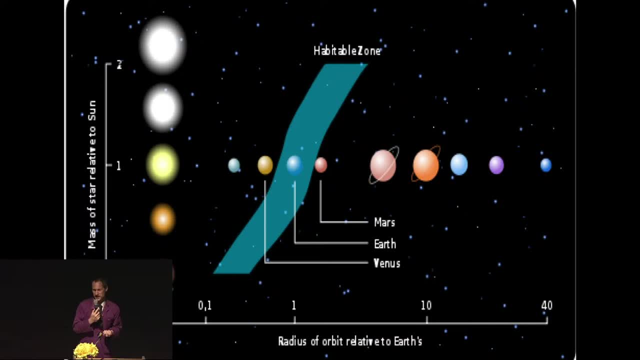 as scientists, we have to bear this in mind all the time. We only have one sample of data about life, because the Earth is the only planet where we know that it's happened, And if you only have one measurement in science, you know nothing at all. Okay, So we always have to bear that in mind. 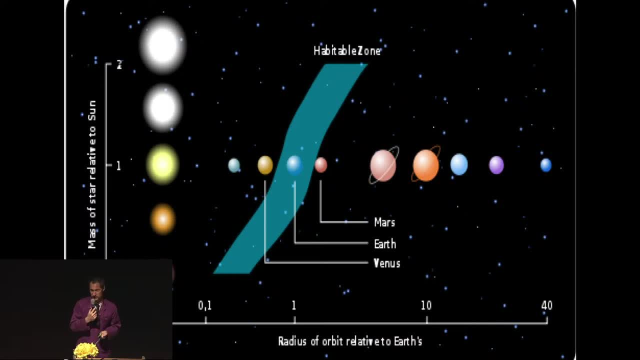 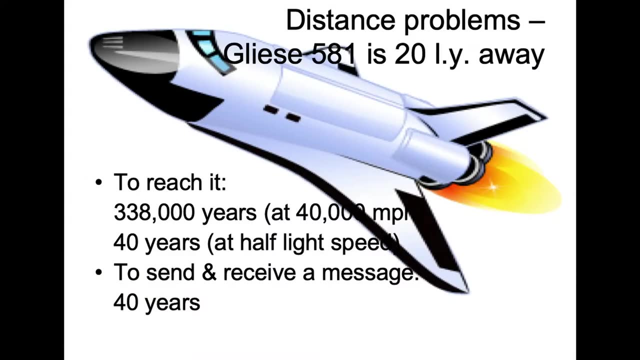 as we're searching, Okay, Okay, we don't really know what we're looking for, Righto? okay, Here's a little idea about those distance problems then. So I mentioned to you one light year nine and a half million million kilometers. 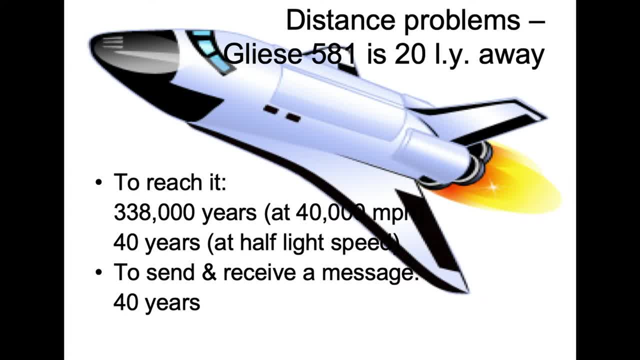 and I chose this star system as an example. Gliese 581 is a system where we know there are, at last count, at least five other planets orbiting that star. okay, And at least one of them is in the habitable zone, okay. 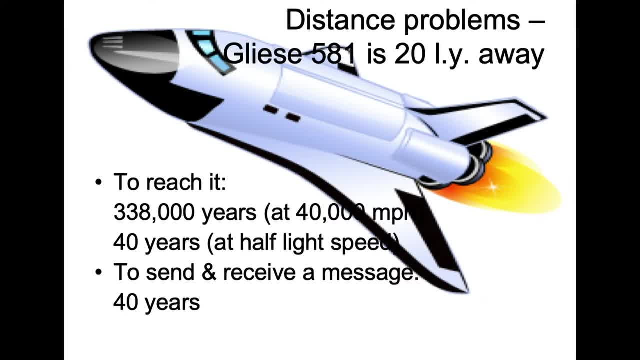 And that's 20 light years away. So if we were to send signals to this planet and there was life and they replied the time it would take for us to signal saying hello. how are you Assuming that they could decode that instantly? 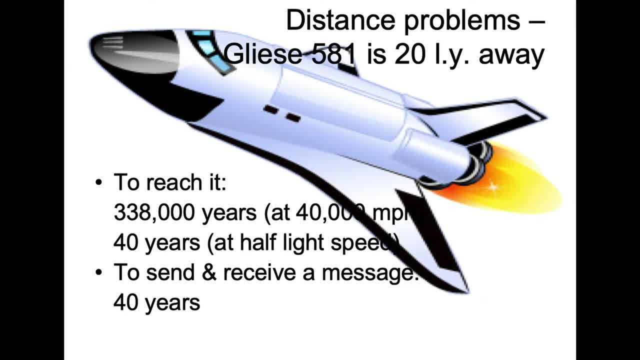 into their own language and reply back saying: hi, nice to see you, let's be pen pals. that's gonna take 40 years. okay, The scientists who send the message are going to be retired by the time the answer comes back. 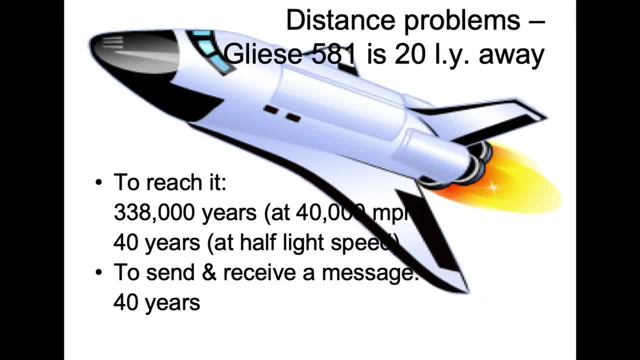 And if we were to consider actually traveling there, even if we could build spaceships that traveled at half light speed, that's gonna take 40 years to get to a system 20 light years away and another 40 years back. okay, 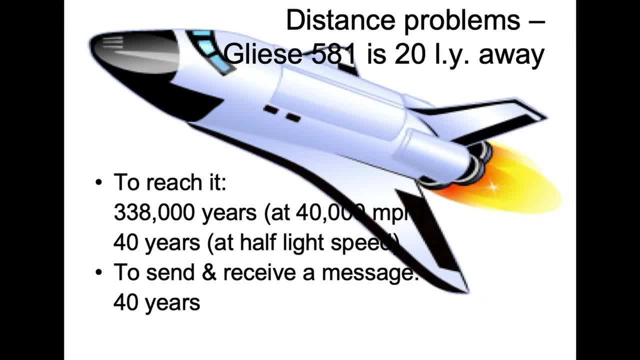 To travel there at speeds we can manage at the moment, say 40,000 miles an hour, that's gonna take 338,000 years. So the scientists who travel on that trip are not just gonna be retired by the time they get there. 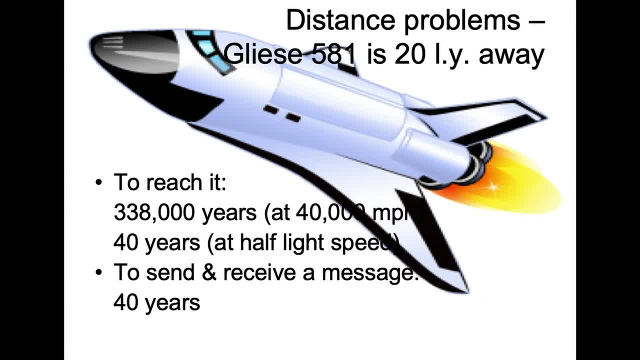 there. They're going to be so dead that if you built a ship big enough to have future generations, their names would probably be forgotten. So it's a big challenge, But there isn't actually any new physics involved in building spaceships that could travel at half. 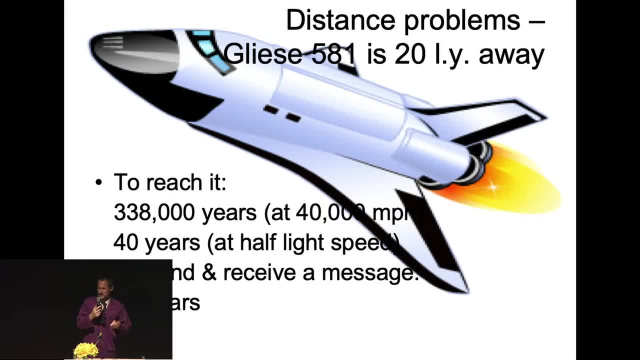 light speed. At the moment it's not a possible technology for us to do with our current economies and what other things we need to spend money on. It would be ruinously expensive, But we know how to do it. So perhaps one day this idea of a 40-year trip becomes within our 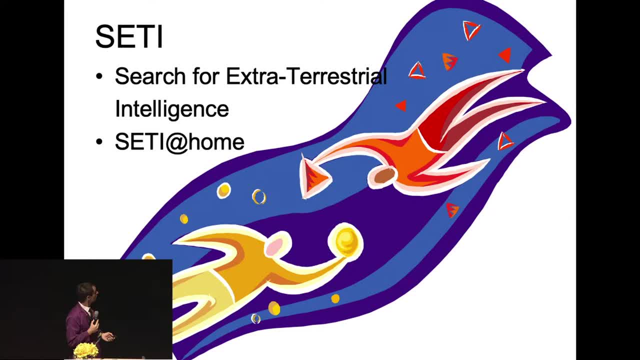 capabilities. Okay, so a bit more about this search, then that Carl Sagan started up SETI, or the Search for Extraterrestrial Intelligence. The whole idea of listening to the radio signals to see what we might hear was Carl Sagan's idea, And he not only made it. 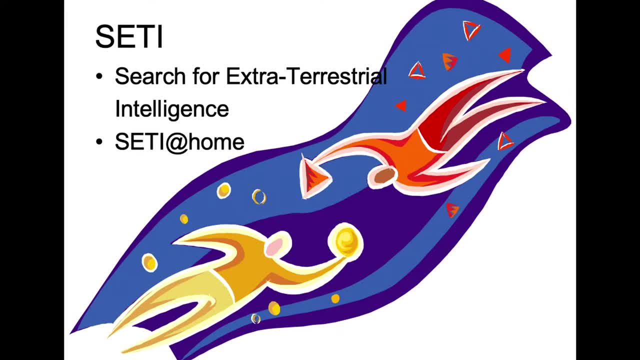 respectable within the scientific community. he started up a project called SETI at Home some of you may have heard of, which was not quite the first but one of the first examples of distributed computing, where a project that requires a lot of computing time and 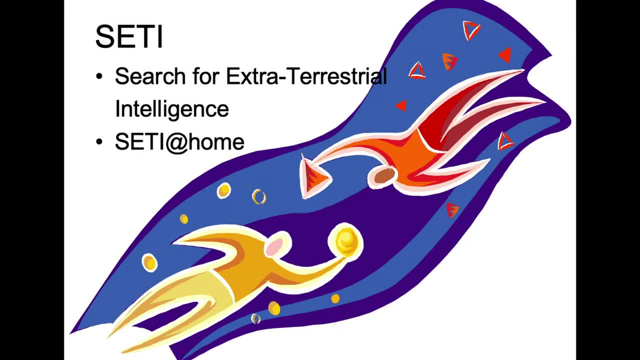 power uses not just the computers in the university- Well you know of the scientists who are working on it- but computing power from people all over the world who are willing to download a program and when they're not using their computers but they're still plugged in to help in analyzing the streams and streams. 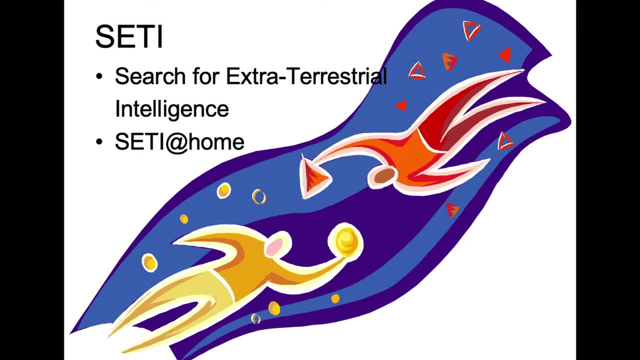 of data that we get into our satellite dishes from all the electromagnetic radiation that's arriving at the Earth. So SETI at Home was one of the first and it really was the most successful in terms of embedding this idea, This idea of distributed computing, in the academic world. That program itself is actually. 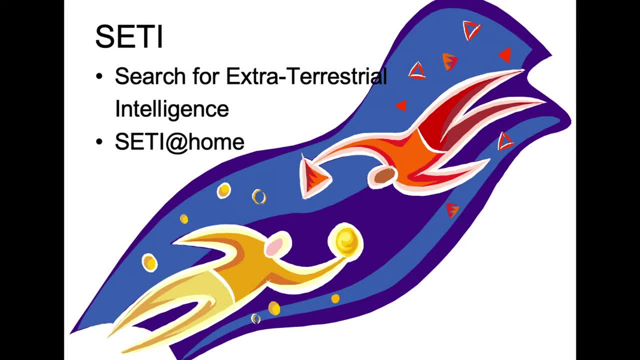 on pause now, but if you're interested in the idea, then there are lots of similar ones. now I run one called Milky Way at Home, for example, which is involved in collecting data to build a 3D accurate map of the Milky Way. There are several others that do a similar. 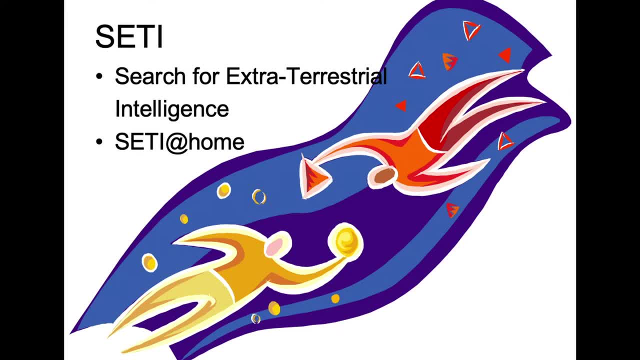 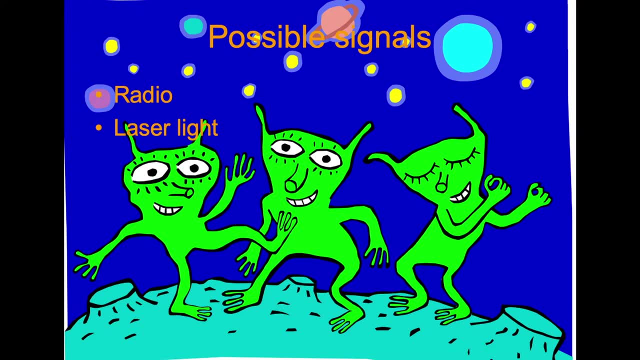 job to SETI. at Home You can investigate them. So what exactly are we looking for? Well, we started off thinking that radio signals are going to be the best ones, because our civilization at that time was very busy. in the radio spectrum We find it very easy. 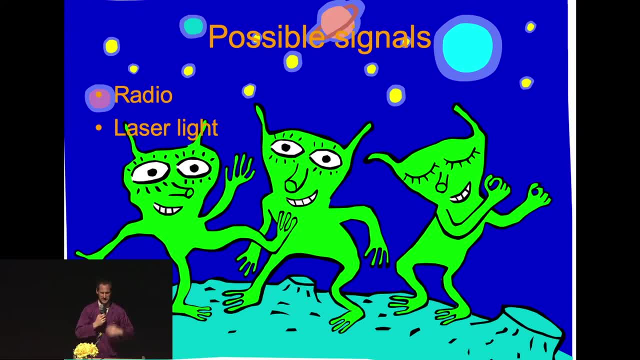 to send signals. that way, We make a lot of noise with our radio and television broadcasts, But actually the amount of stray radio noise that Earth civilization emits into space has decreased a bit now since the 80s and the 90s, And so we start to wonder whether an 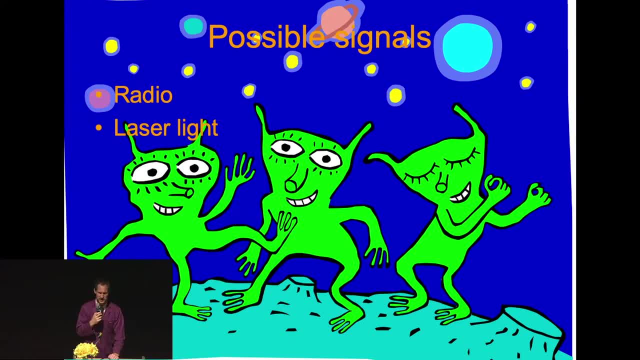 advanced civilization actually won't be emitting much radio. One other possibility that some scientists think we ought to be looking for is laser signals, which are just as good at propagating through tens- hundreds of light years and are far easier to direct accurately. This is a possibility for the near future. 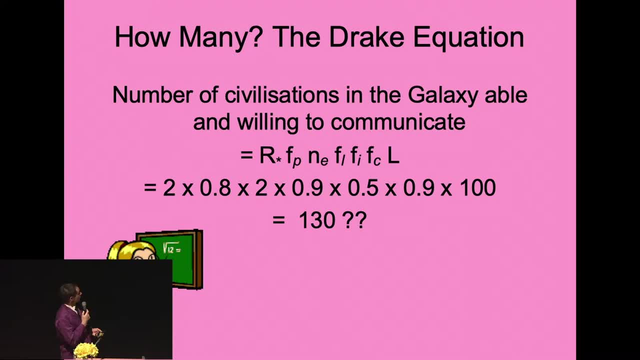 So I warned you, there was an equation. The wonderful thing about this equation is that really that it's nonsense. We don't know any. well, that's not quite true. We don't know very many of the numbers that those symbols represent accurately at all. When Frank Drake came up with 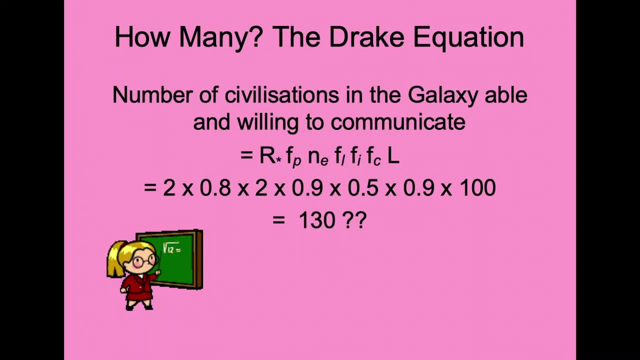 this equation. he didn't mean it as an accurate way of estimating how many other life forms or how many other civilizations there are in the galaxy. He meant it as a basis for discussion. Look, these are the kind of things we're going to need to know, okay, So please remember, this is. 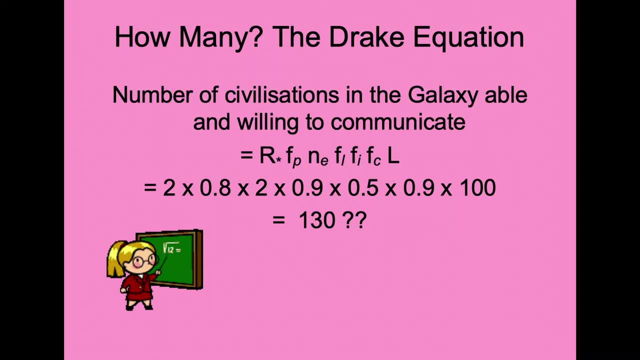 not going to give us a nice answer, but the equation says that. well, you can read what we're trying to get there. and on the right-hand side of the equal sign, R star represents the rate of star formation in the galaxy. okay, And at the moment our best guess is that's approximately. 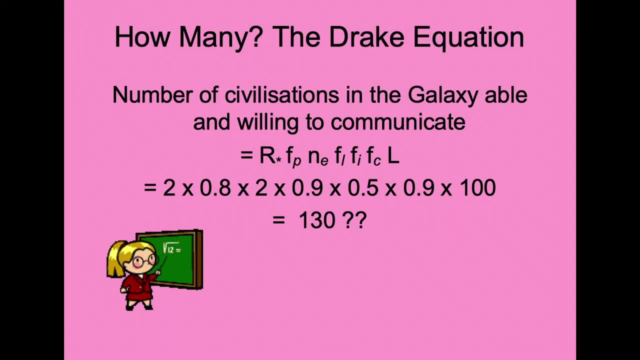 two per year. On average, about two new stars are formed per year. okay, FP, what fraction of those stars have planets? Okay, and of course, back before the first exoplanets were discovered, you could argue that that was zero. We now think it's actually far more common for stars to have planets than not to. 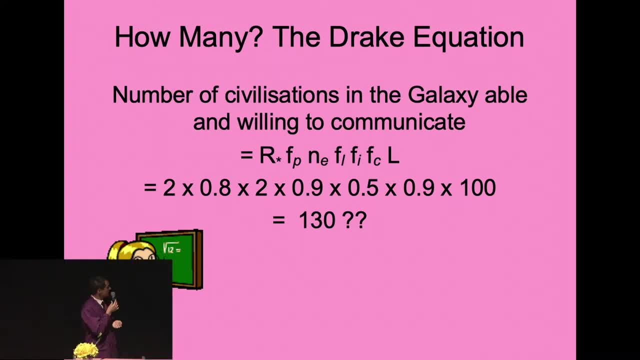 So perhaps 0.8, 80% of stars have planets. NE. how many planets does an average star system have, if it's got any at all? okay, Again, this is really guesswork. 4,000, 4,500 exoplanets, I told. 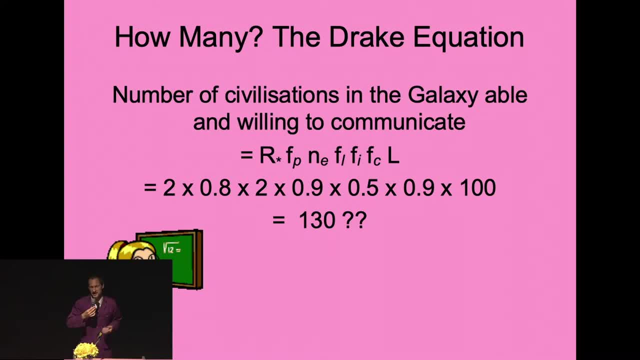 you, we discovered That doesn't really give us enough data to put in an average. Let's say two FL. if you've got planets, on what fraction of them does life develop? This is the most controversial fraction in the equation because, as I said earlier, we only 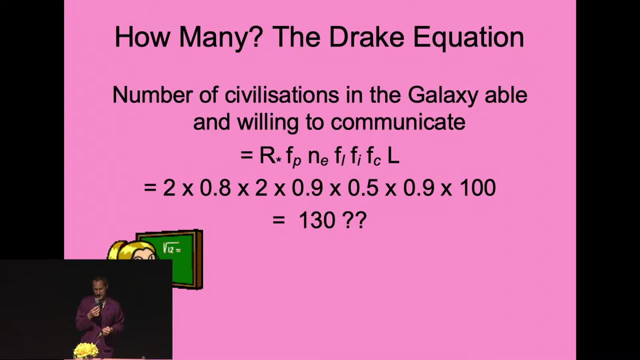 have one data point: Earth is a planet where life might develop, and it did So. some scientists say that number should be high. I put it in as 0.9, 90% chance that if life could develop, then it will. 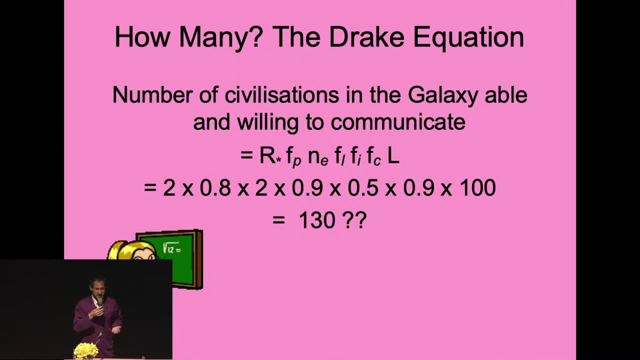 If I once life develops, does it go on to be intelligent Again? we don't know. It did on Earth, but only once. Only Homo sapiens sapiens became intelligent out of all the billions of species that have ever existed on Earth. So you could argue that it's an extremely unlikely thing. 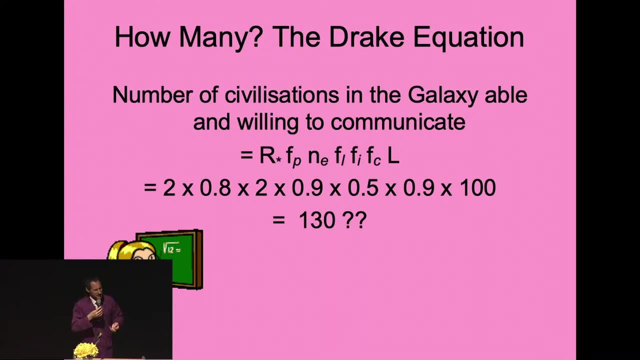 to happen. or you could argue that well, it's happened once and we've become masters of this planet and we're not about to allow others to do it, So it's an extremely unlikely thing to happen. You could argue that it's happened once and we're not about to allow other species to evolve into. 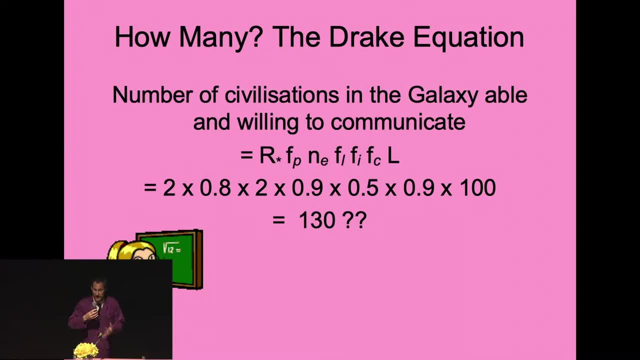 intelligent life. Or you could argue it's happened to us already after only a few billion years of existence of the Earth. If you waited a few more it would happen again and again. So again, very hard to put a number on that. I've stuck it in as a 50% chance FC once you've got intelligent life. 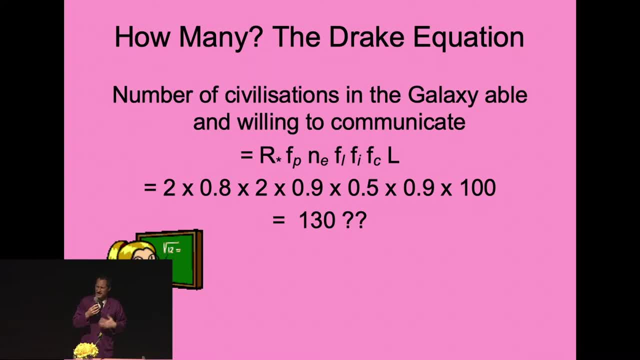 would they become willing and able to communicate? I think able kind of comes with being intelligent, but would they want to? Would you want to If you knew there were definitely other technologically advanced civilizations out there? would you want humanity and the Earth to enter into contact with them? Or? 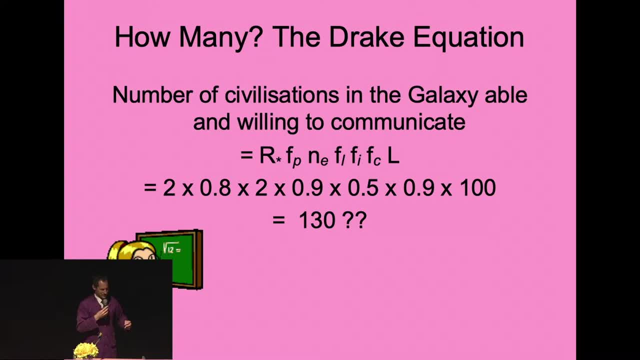 would you say: no, better not- we don't know if they're friendly- Or build a defense system just in case chatty civilizations come and we want them to go away. Again, we have no idea, Maybe 90% of them would want to. And finally, once you've got a civilization which is willing and able to, 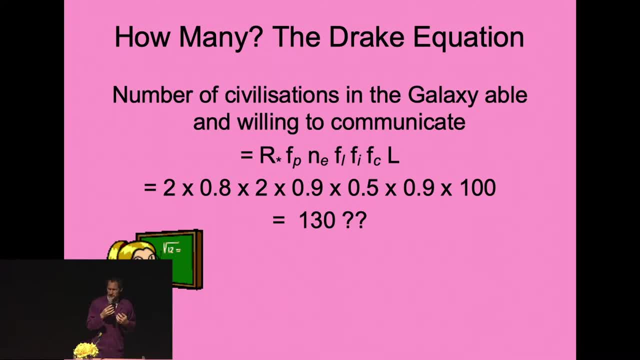 communicate. how long does it last? When Frank Drake made this equation, the United States and the Soviet Union looked pretty likely to blow up the entire planet in a nuclear war very soon. So 100 was perhaps the length of time they thought that human civilization was going to exist before we. 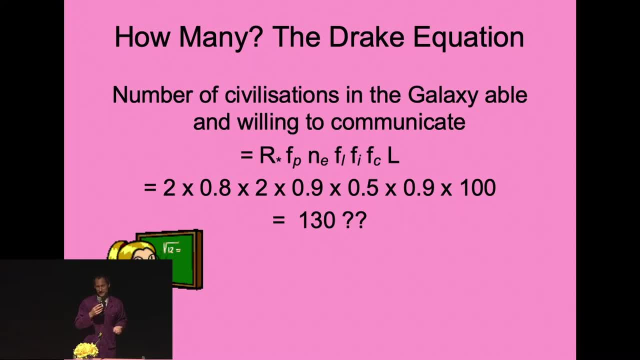 blew ourselves up. The specter of nuclear war and cataclysm has perhaps receded a bit since then, although the major powers of the world have not yet been able to do so. So I think it's a good idea to think about nuclear war and cataclysm, because nuclear wars still have too many nuclear bombs. So you 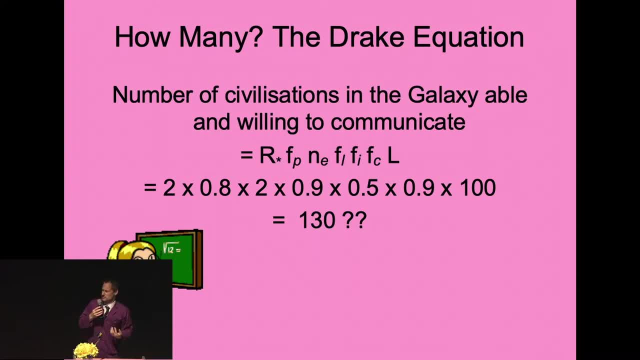 could argue, perhaps, that every civilization would be as lucky as we were to avoid nuclear war and they'll last for 100,000 years. So that last number is also not accurate in the slightest. So basically, with all those unknowns, you can justify an answer to the Drake equation of pretty much zero. We are. 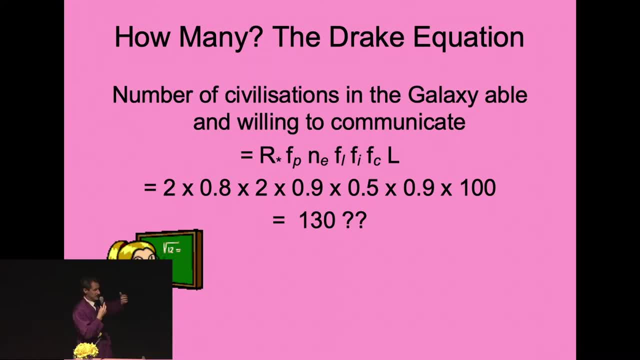 alone in the galaxy And you can justify an answer of several hundred thousand years, And you can justify an answer of several hundred thousand. We should be able to discover alien life before very long. So it's just an equation to get you thinking about the sort of factors that affect the chance rather than 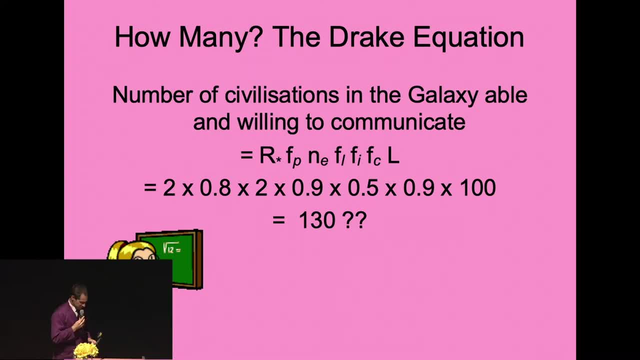 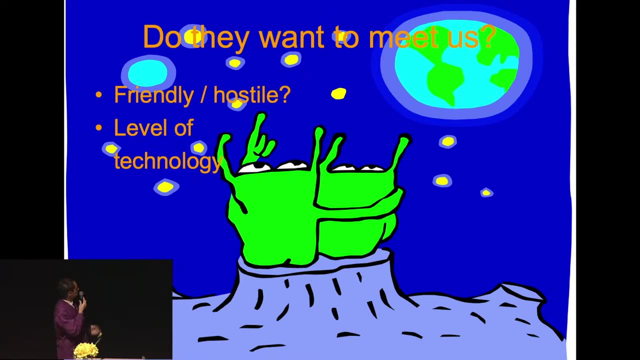 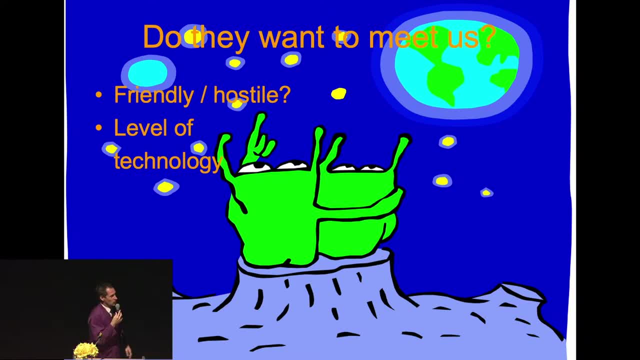 ruled by an evil empire with Darth Vader and the rest of it? Or will we find that alien life wants to be helpful and aid us in our technological progress? We have no idea. Will they even want to talk to us? Would a space-faring civilization perhaps look on us the same way we look on 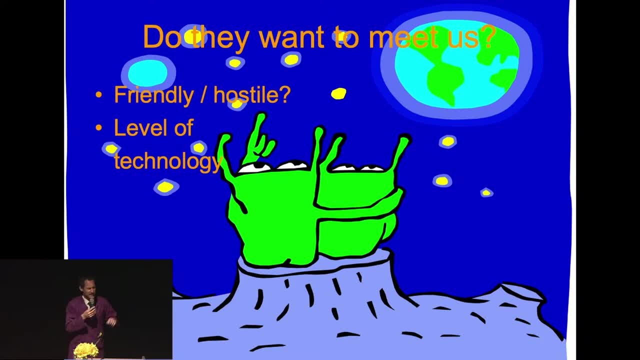 monkeys. If you're a specialist in monkeys, well they're fascinating and you're happy to spend your whole life studying them, but most people just ignore them. Maybe that's how we will appear to other civilizations. Only specialists would show any interest in a backward bunch like us. 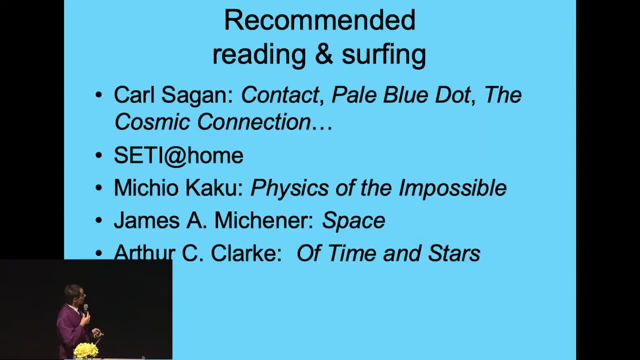 whatsoever. If you've been interested, here's a little recommended reading and surfing for you. As I mentioned, SETI at Home is paused, but there are other similar projects out there. Some of the original books by Carl Sagan are well worth reading. His ideas about space flight. 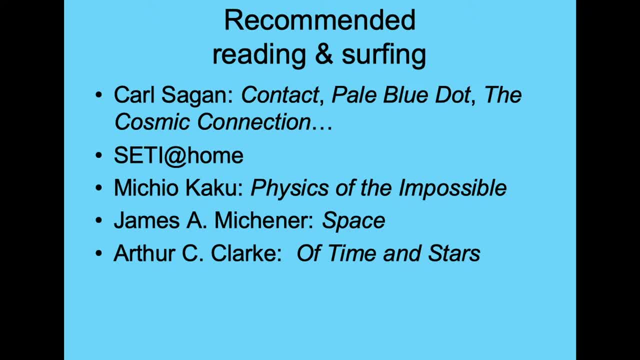 are a bit dated now, but his ideas about what we call terraforming, about how we can change the world, about how we can change the world, about how we can change the world, about how we might one day make other planets like Mars and Venus habitable for us. 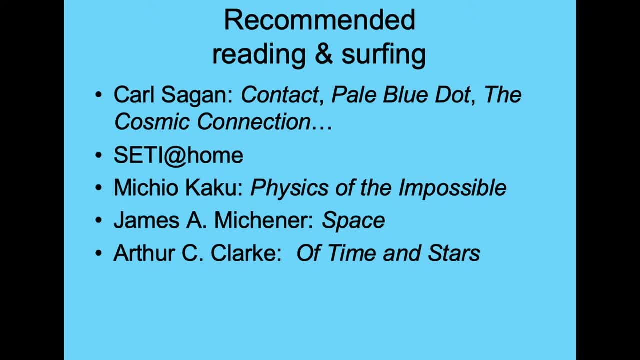 have not. They're still very much on the money. Michio Kaku is a respected theoretical physicist who talks a great deal about how physics is going to evolve, what things that are technologically impossible now are likely to become possible within 100, 1,000, 10,000 years. It's in the